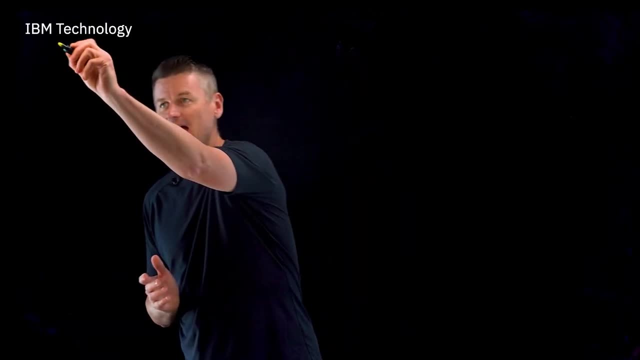 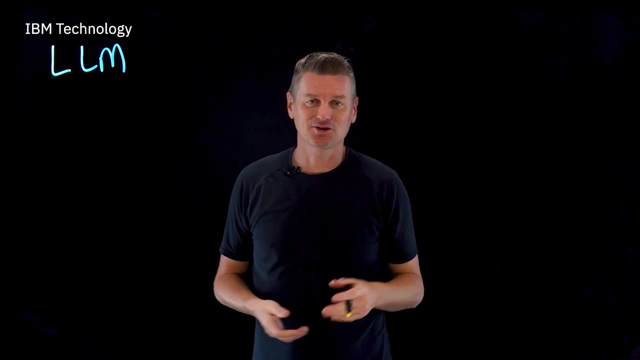 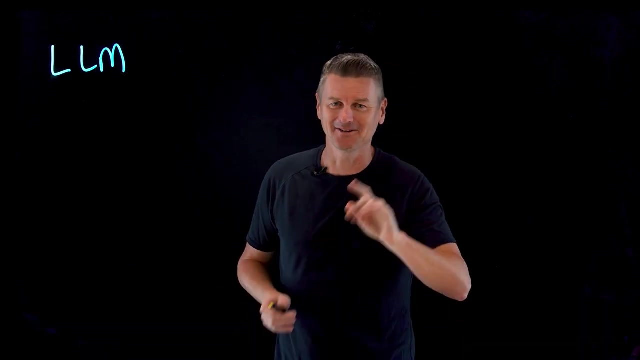 If you're not getting the responses you want from LLMs or large language models like the model that powers ChatGPT. I may know what's wrong. It might be you. No, no, no, hear me out. hear me out. You see, the way that we prompt these large language models is very. 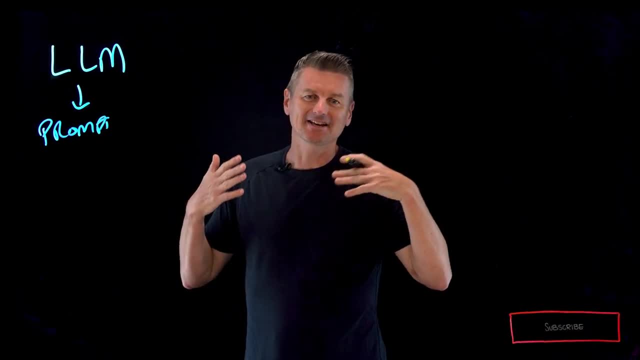 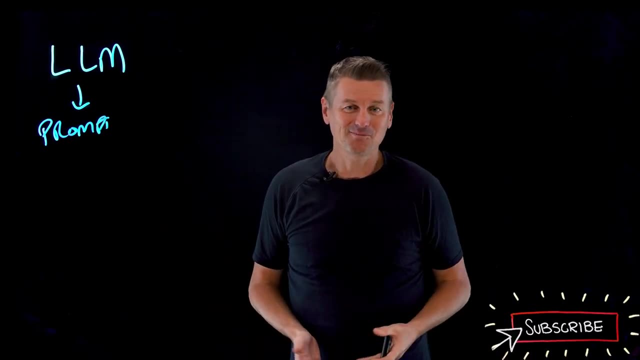 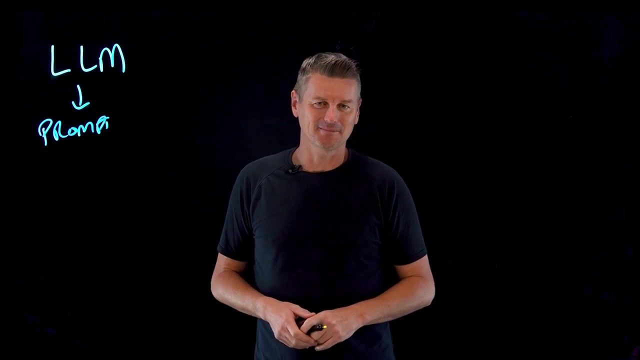 important, So prompting plays a significant impact in the quality of the response that the LLM will generate. Let's take a look at an example. I'm working on a homework assignment for my Econ 101 class and I need some help, So I issue the following prompt to a large language: 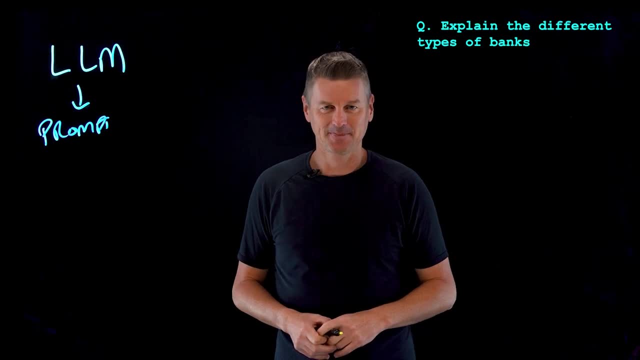 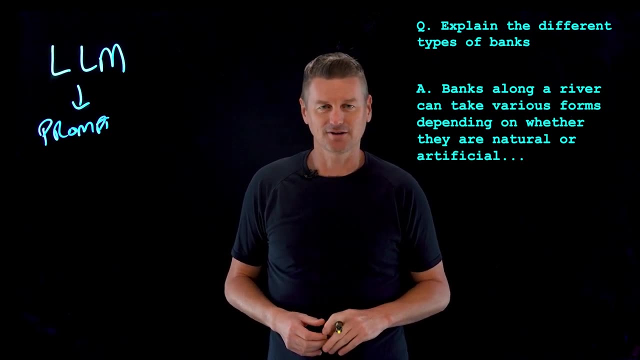 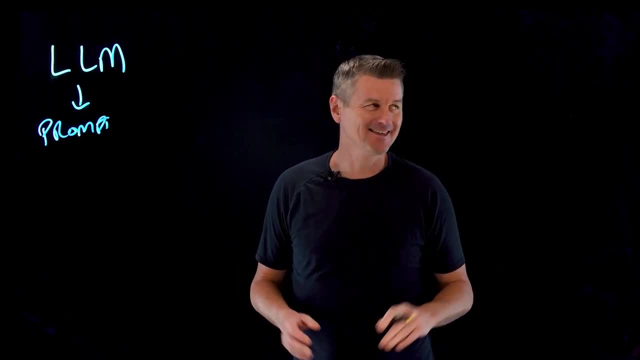 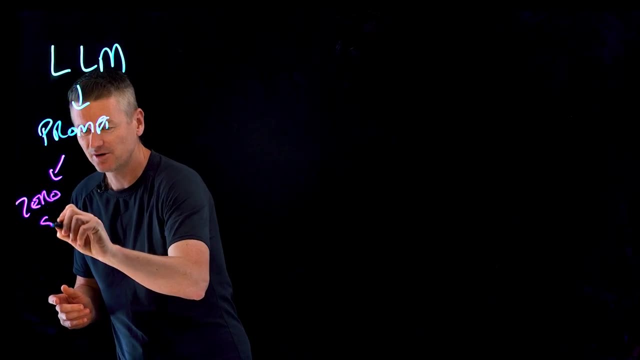 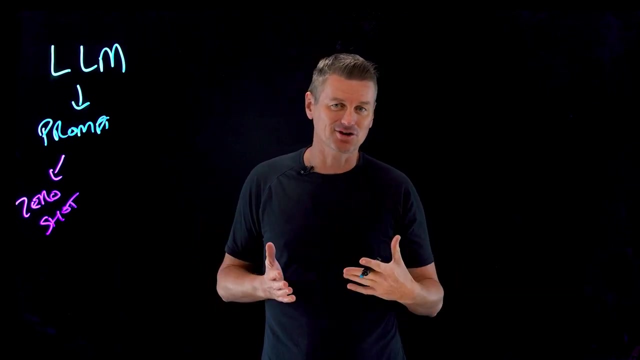 institution And it's talking to me about river banks. This is an example of a particular type of prompt, and that is called zero shot prompting. You're providing the model with a single question or instruction, without any additional context, examples or guidance. The model is expected to 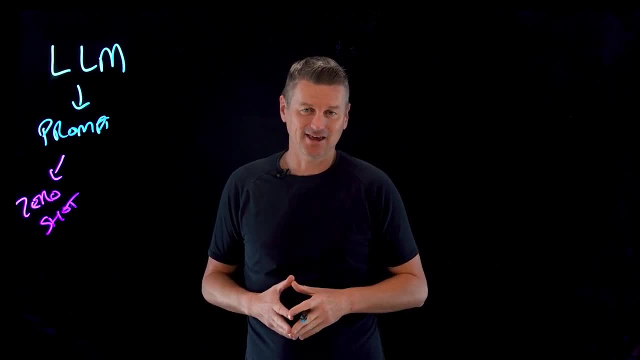 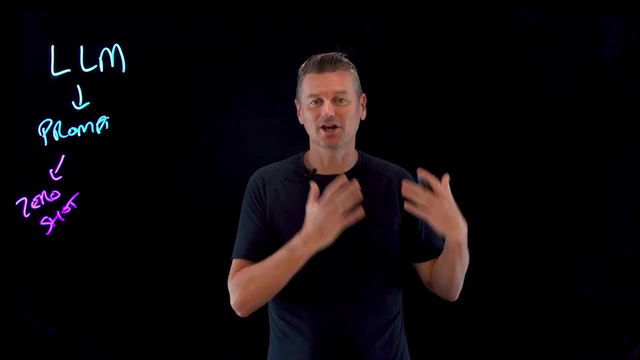 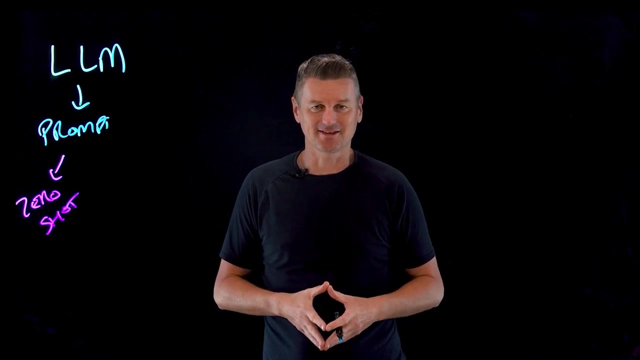 understand and answer the prompt without that context, And to do so it relies solely on its pre-existing knowledge and its ability to generalize from that knowledge to generate a relevant and accurate response And, as you can see, it can lead to some suboptimal responses. Now, bank is a homograph. It has 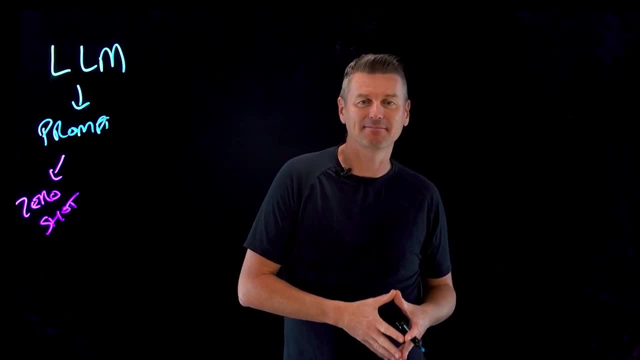 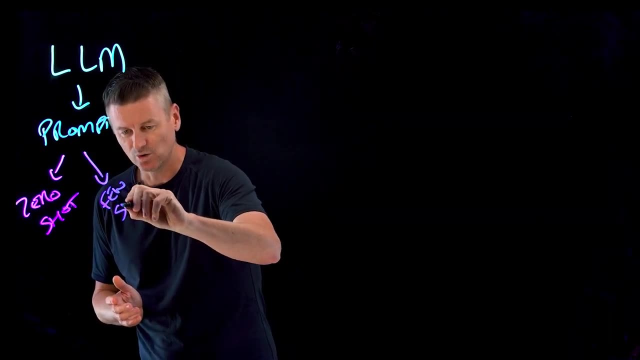 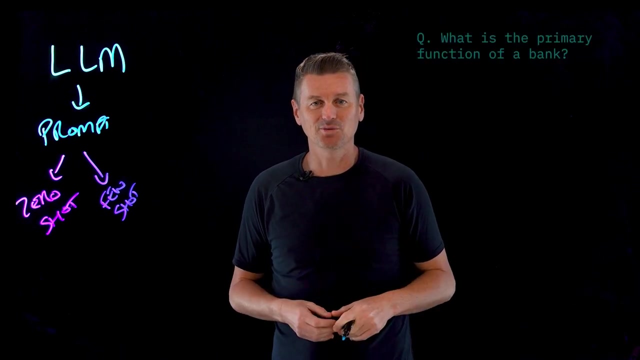 multiple meanings. One method to clear that ambiguity up is to employ a different type of prompting called few shot prompting. Now here is an example of few shot prompting. So we've got question: what is the primary function of a bank? Answer: a bank's primary function is: 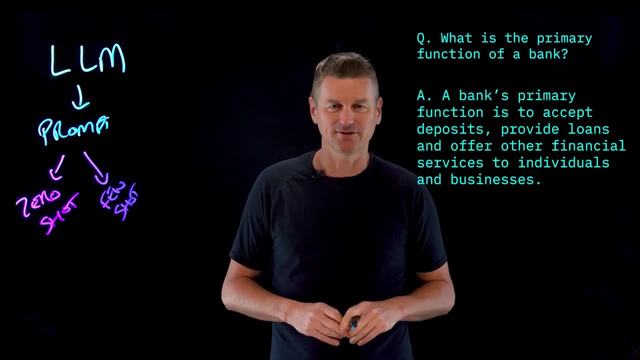 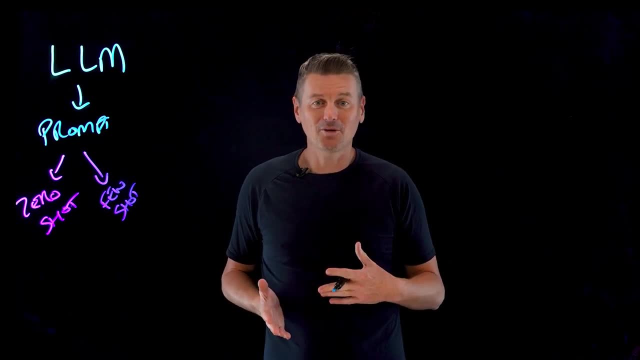 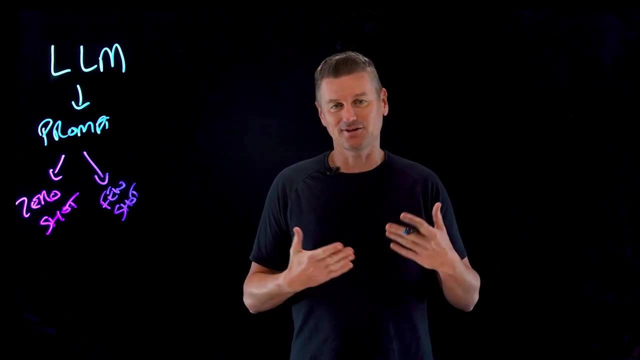 to accept deposits, provide loans and offer other financial services to individuals and businesses. Question: explain the different types of bank. With few shot prompting, the model is provided with one or more examples to help guide its understanding of the task at hand. By providing an example related to financial institutions, the LLM. 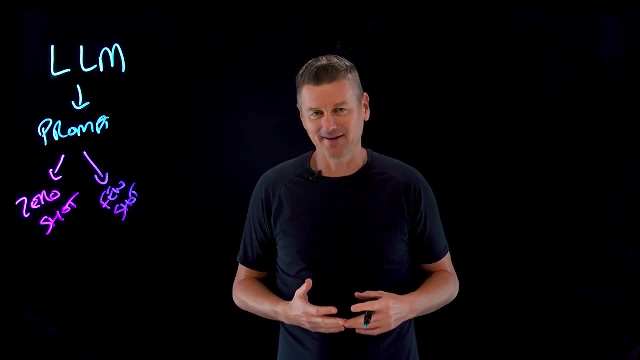 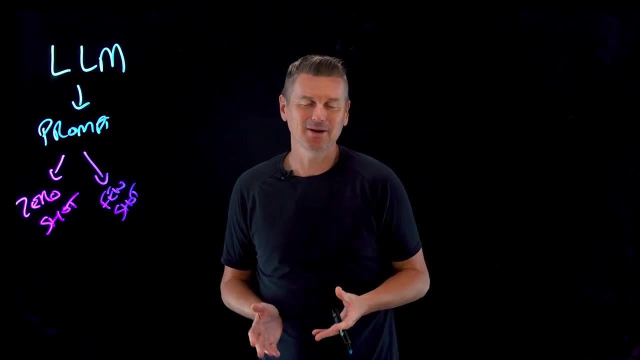 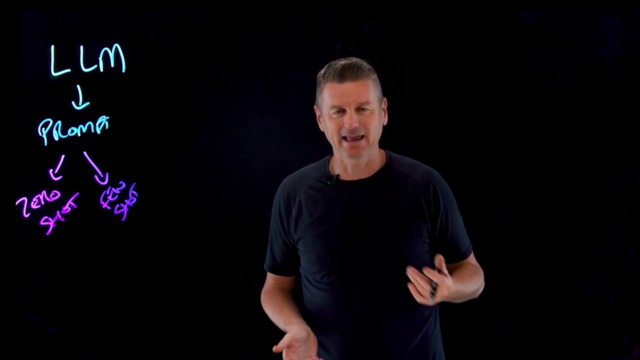 is more likely to understand that you are asking about types of bank in the context of finance, rather than the stream at the bottom of your garden. Now, in this example, we could probably just have used a better zero shot prompt, like: explain the different types of banking, financial. 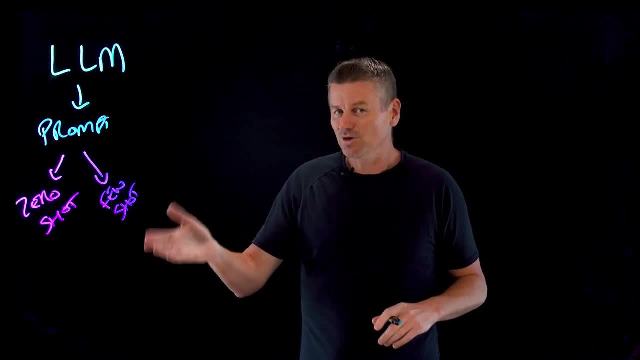 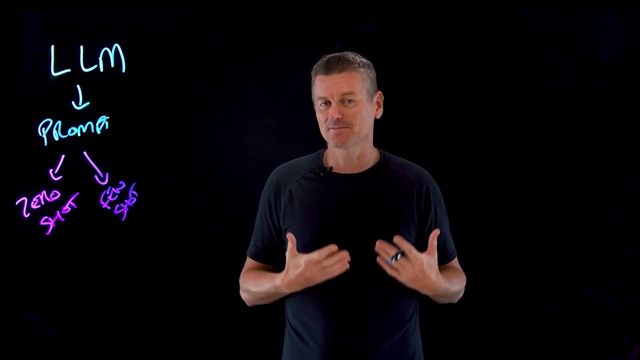 institutions. That probably would have worked, But few shot. prompting has other advantages too. It can help an LLM understand the expected format. a response should take like this: So we've got question. create a title for my web page then. 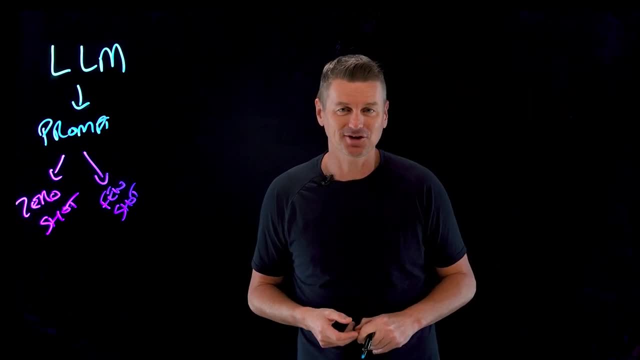 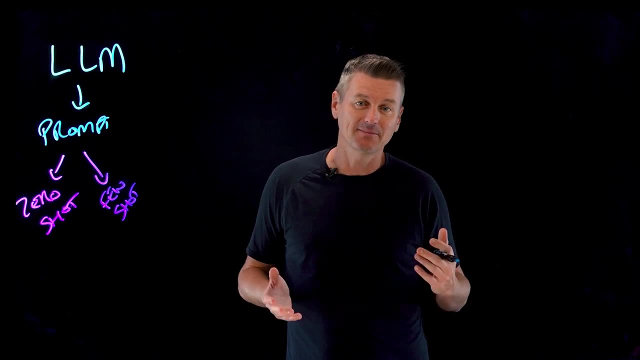 a title tag with all about banks, then question: create a heading for my article. Then we have an H1 title pair with types of banks in those tags And then we say question: list the types of banks. And here the LLM may derive. we are looking for answers in. 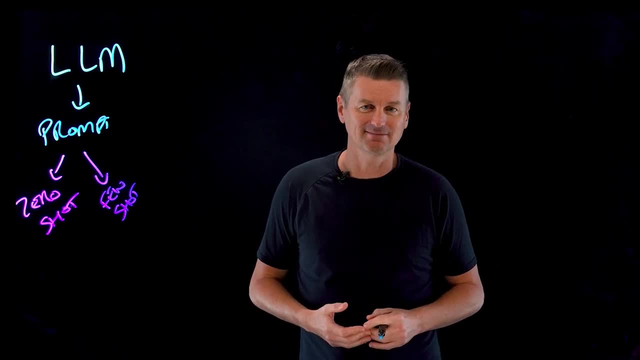 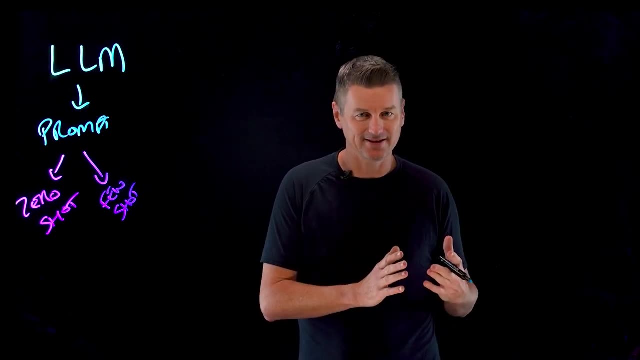 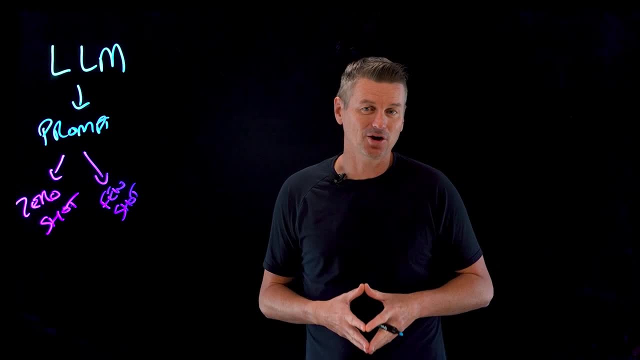 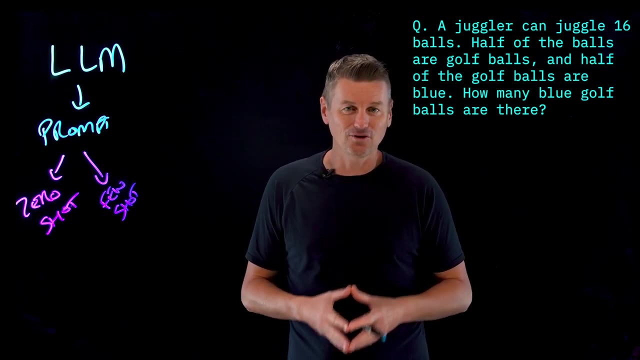 page that we're looking at. So let's take an example from the page that we're looking at. And they issued this zero-shot prompt to a large language model Question. A juggler can juggle 16 balls. Half of the balls are golf balls and half of the golf balls are blue. 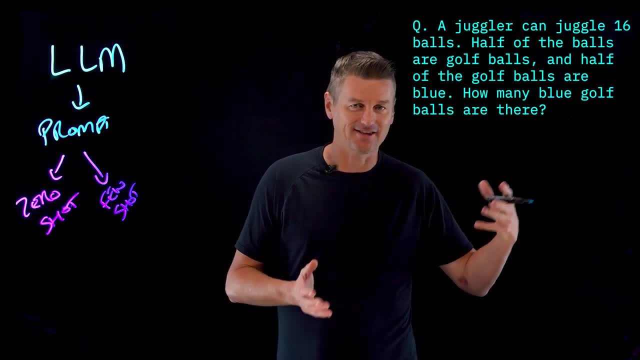 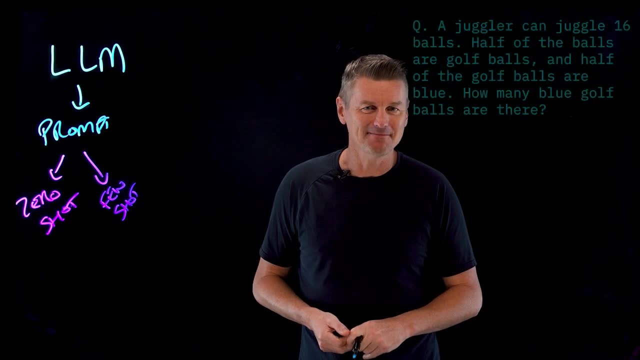 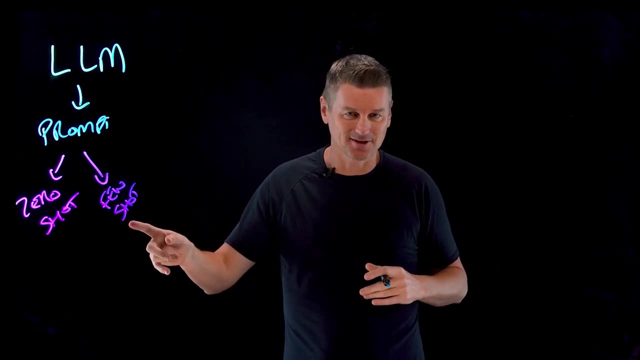 How many blue golf balls are there? The answer is Now. can you figure this out? It's not too tricky, but it was for the LLM 8. Wrong, So next in the paper they tried a few-shot prompt. 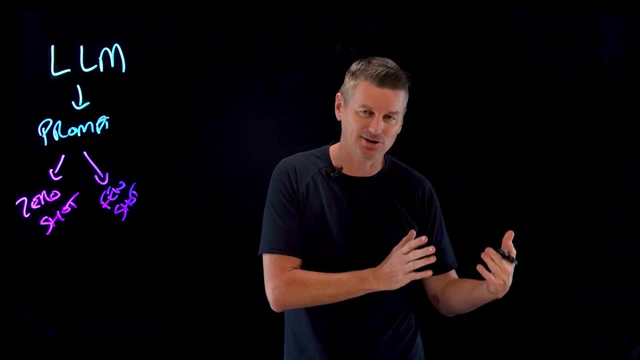 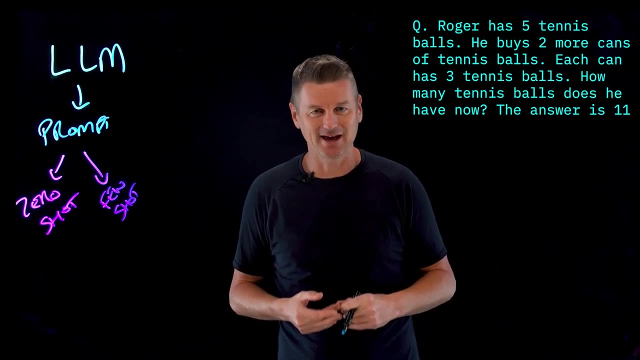 So we start off with a sample question and a sample completion. So question: Roger has five tennis balls. He buys two more cans of tennis balls. Each can has three tennis balls. How many tennis balls does he have now? Answer: The answer is 11.. 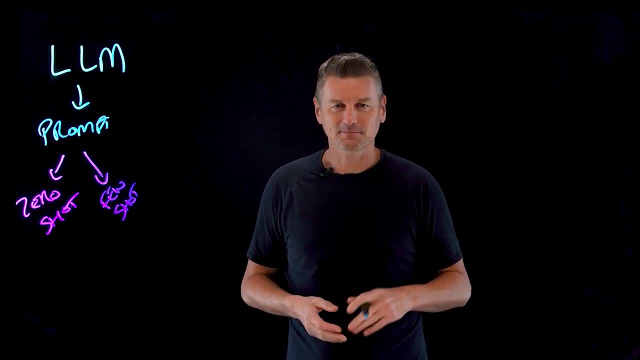 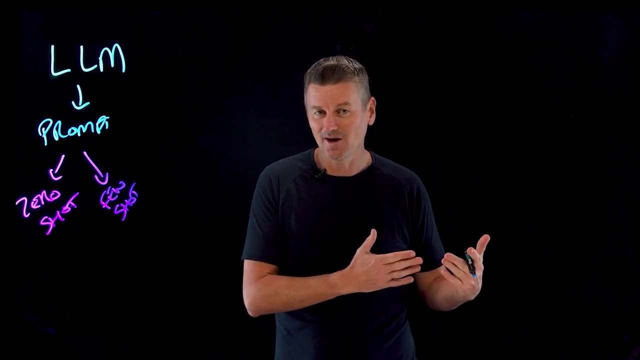 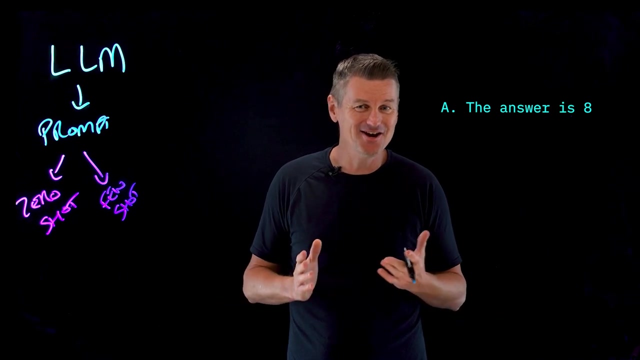 Question: A juggler can juggle 16 balls and so forth. Now we've shown the model what a right answer looks like by applying addition and multiplication to a sentence. So did the few-shot prompt get us the right answer? 8 again no, but by making a slight change. 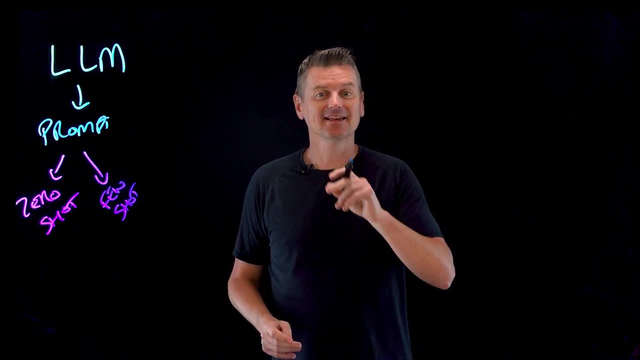 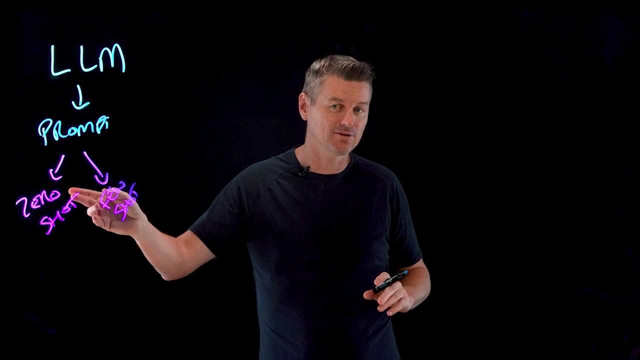 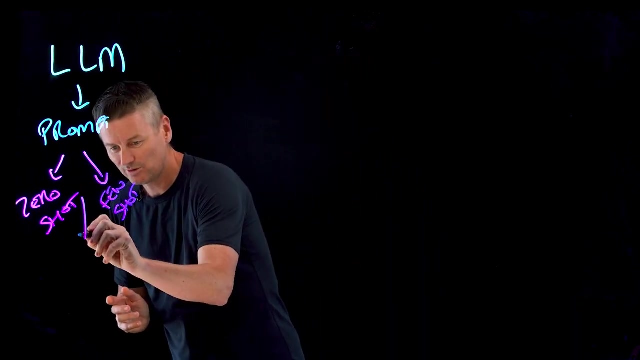 we can improve the reasoning of the LLM and get the right answer, And we can apply that change to either few-shot prompts or to zero-shot prompts. So what is this mysterious addition? Well, it's called chain of thought. So what is chain of thought? 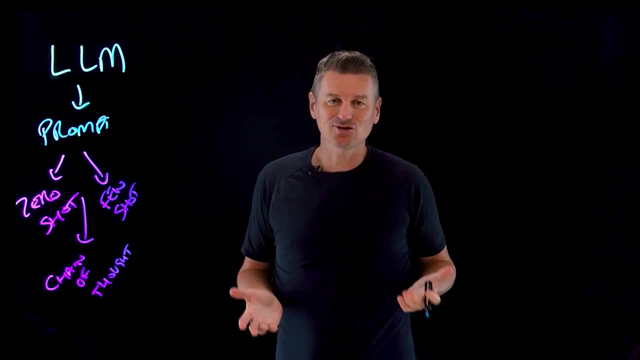 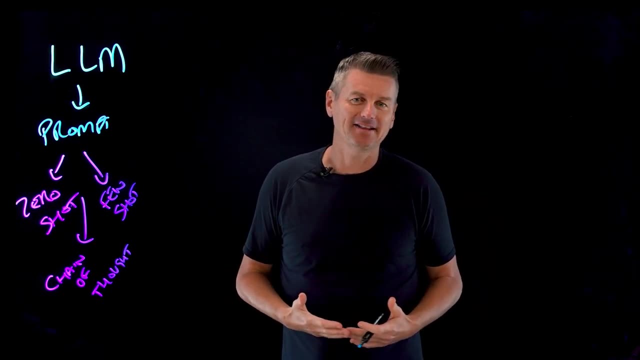 Well, it's called chain of thought or C-O-T And, to invoke it, just add wording such as: let's think step by step. Effectively, we've asked the LLM to document its thinking. We're asking to see its chain of thought. 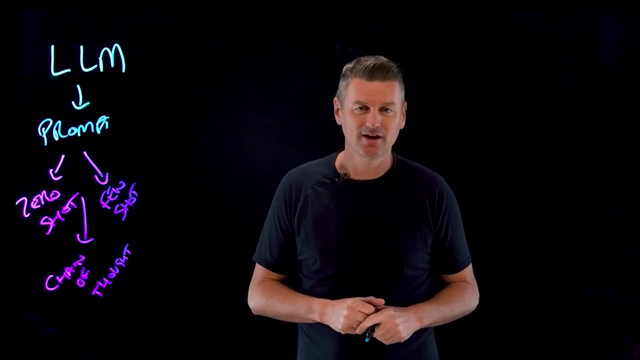 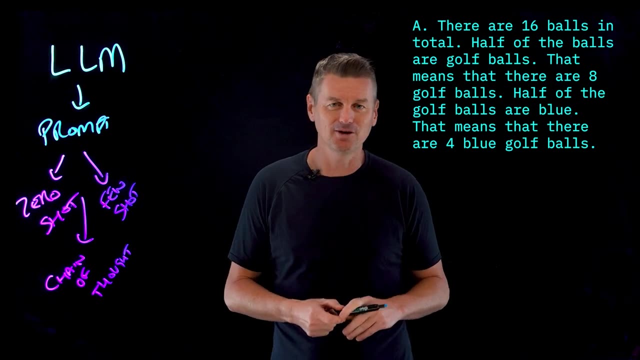 And here's what we get. So the LLM responds to us with: there are 16 balls in total. Half of the balls are golf balls. That means there are eight golf balls. Half of the golf balls are blue. That means there are four blue golf balls. 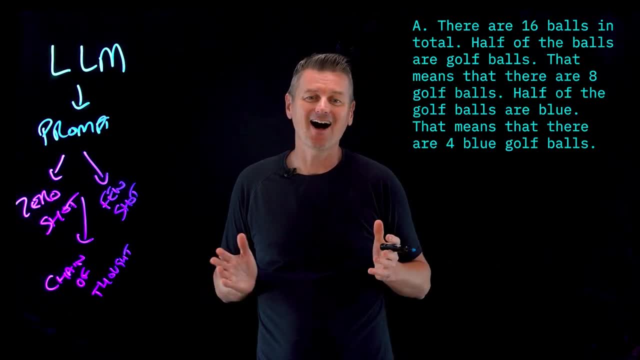 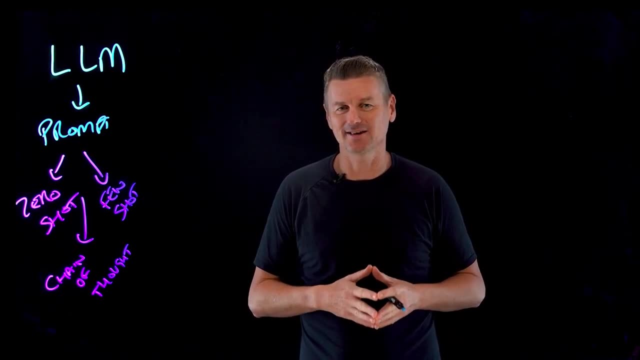 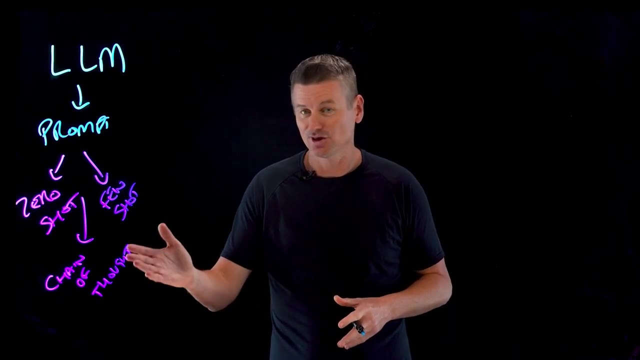 Four golf balls. That is the right answer. Now, this particular test was applied to the Instruct GPT model, which is a couple of years old. Newer models, like GPT-4, can invoke mathematical reasoning without the- let's think step by step- chain of thought prompting. 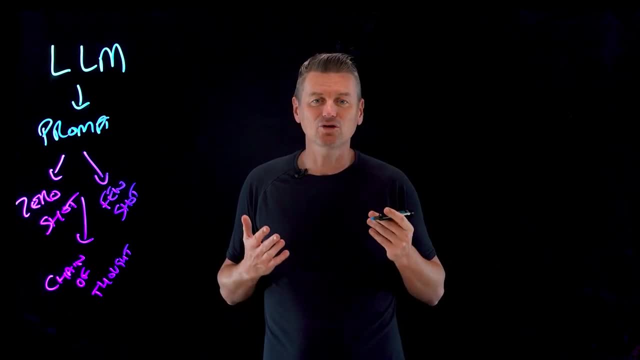 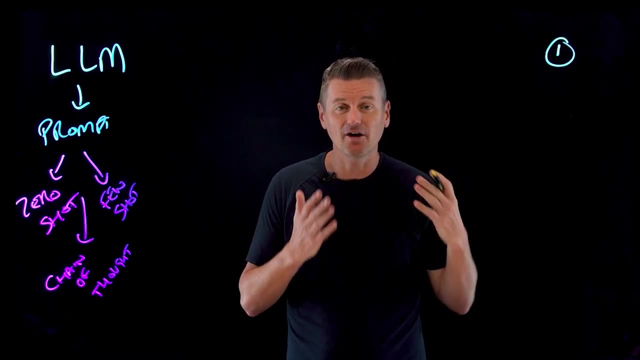 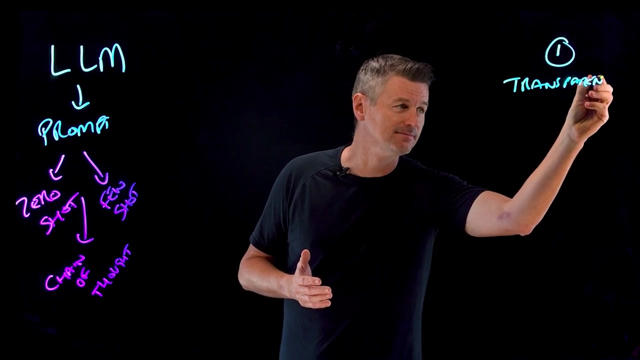 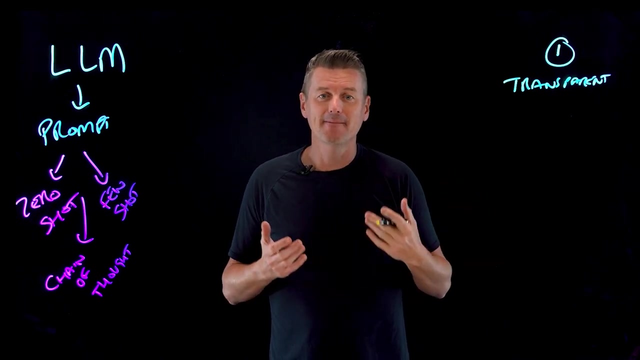 But chain of thought prompting remains a valuable tool in prompt engineering for a number of reasons. Reason number one is it encourages the model to provide a more detailed and specifically, a more transparent response And an explanation of that response and its reasoning process, And this helps users better understand how the model arrived at a particular answer.